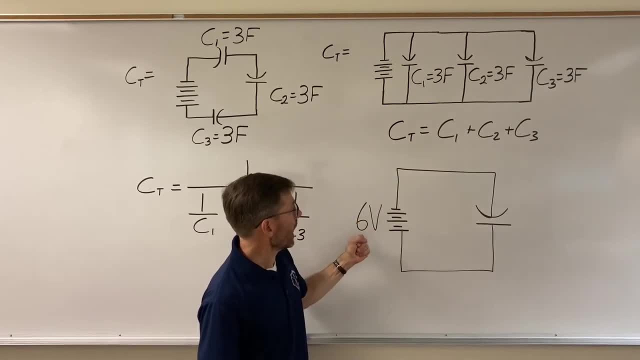 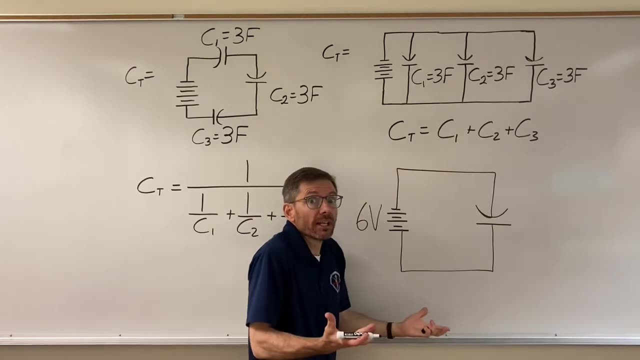 The circuit's closed. So what's going to happen? The battery is going to push some electrons. That's what batteries do: It's going to push some electrons. And where are they going to go? They're going to stack up on this side of the capacitor. Can they go through? No, because there's an 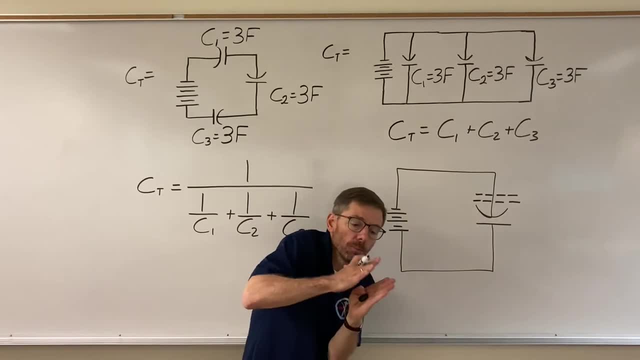 insulator, a dielectric in between the two plates of the capacitor, And so the electrons will stack up here and they will cause the electrons on the other side to run away. Negative repels negative And these electrons are going to get sucked by the positive side of the battery And basically, 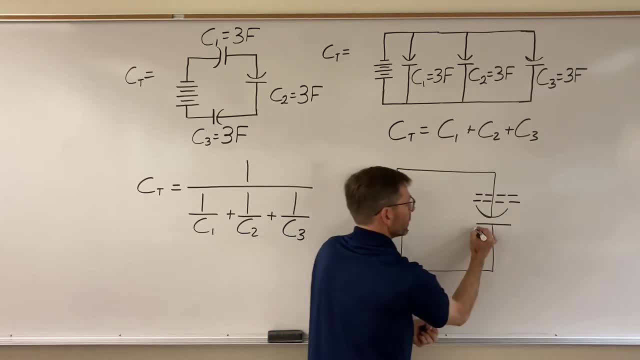 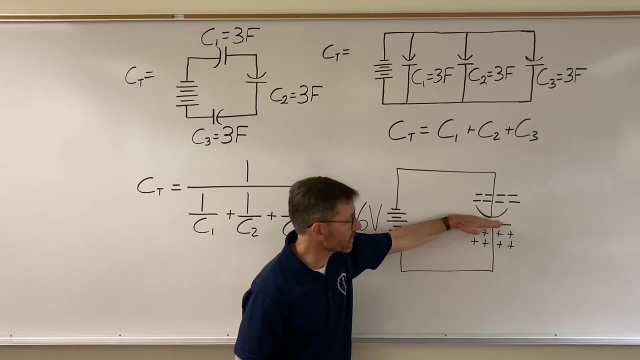 we've got a mass transfer of electrons to one side and the other. When the electrons leave town, we're left with a positive Charge there, Okay, And the characteristics of the dielectric can either encourage a greater charge or they're more apathetic about it. So how long will this happen? How many electrons will flow? 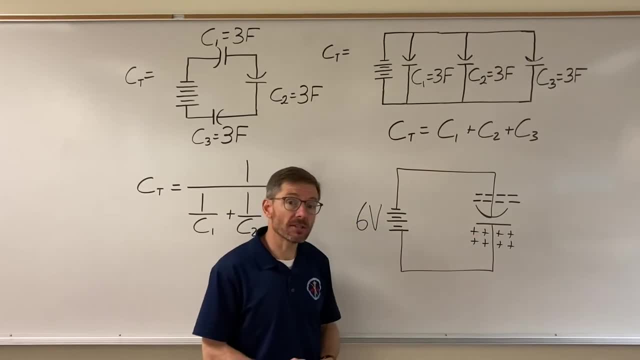 there. Well, until the capacitor gets an equal and opposite charge, Once enough negatives are built up on the top and pulled away from the bottom, this thing builds up an electrostatic charge, And that means a voltage, And its voltage is going to. 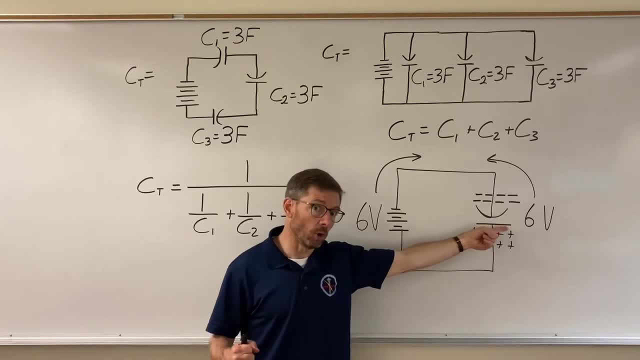 push back Once this gets up to six volts. now the two are pushing at each other with six volts each And there's no more electron flow until we open the circuit or let them release through another load. Okay, But how many electrons can actually stack there? Well, I talked about the 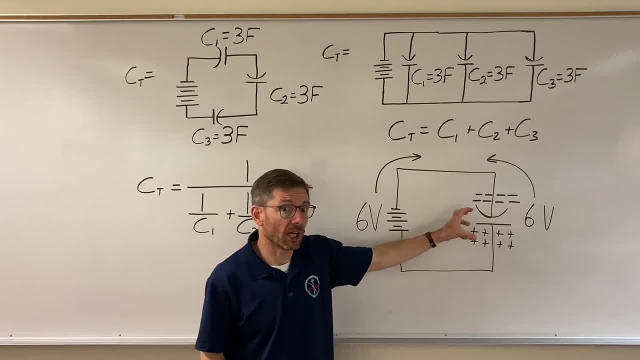 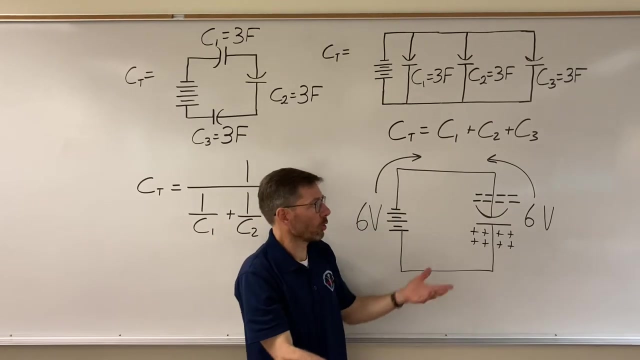 dielectric, whether it encourages a greater charge or not. Okay, And the electrons don't actually go through the dielectric? If they did, it probably means I used the capacitor with too low of a voltage rating and the pressure of the source pushed its way through, therefore causing leakage. 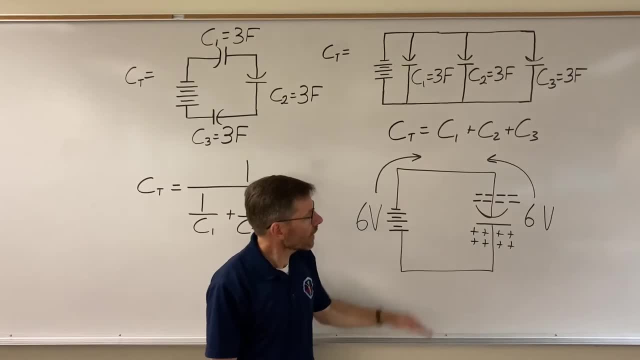 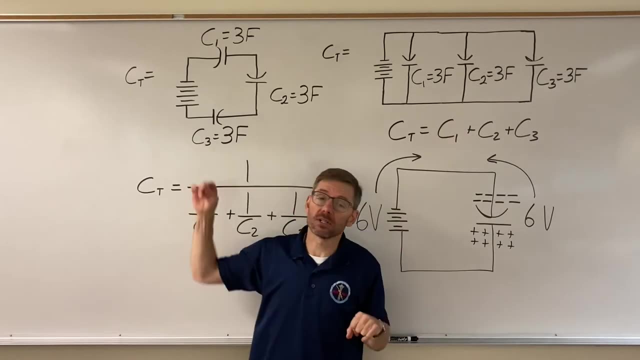 current and shorting it out. essentially Okay. So the dielectric makes a difference, But here's the other two issues we're going to focus on. when looking at parallel and series circuits, The dielectric is the size of the plates. The bigger the plates, the more electrons you can store. 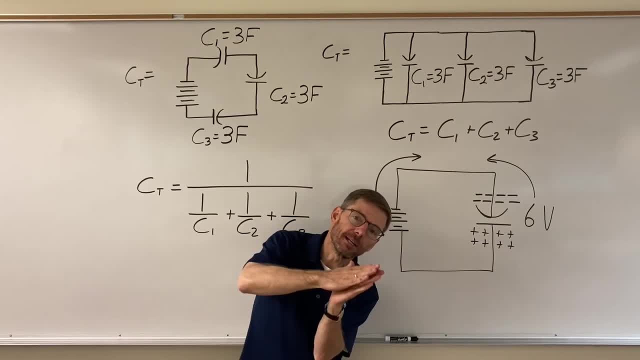 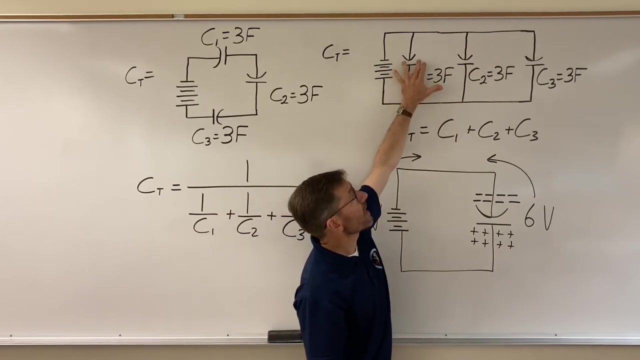 there and the gap between them. As the gap gets bigger, the capacitance goes down. So let's look at our circuits. What's happening here? If I have a voltage source pushing electrons, I'm going to stack some here, stack some here and stack some here. Are all branches getting the? 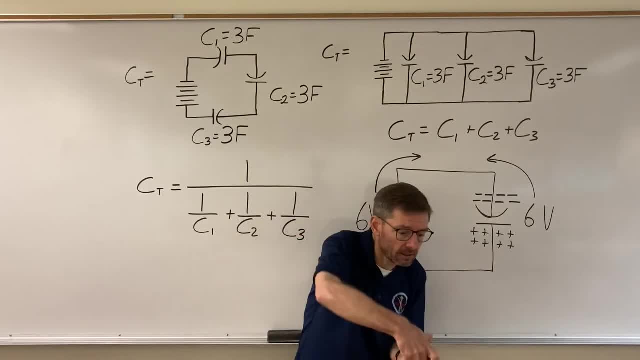 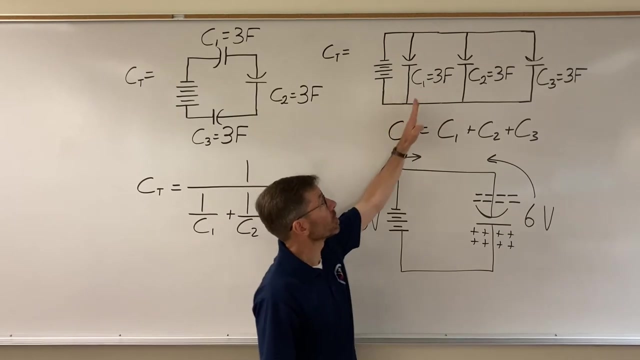 same voltage? Yes, So is it going to stack a bunch of electrons in each branch, And if I add another branch I'm going to add more electrons? Yeah, So you think, well, I should have more of an electrostatic charge, because I've got a charge here pushing back with the same voltage as the 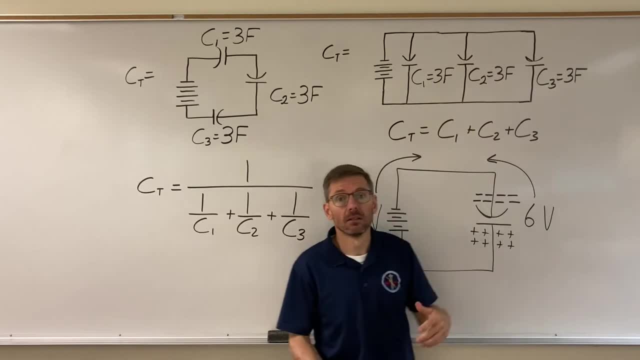 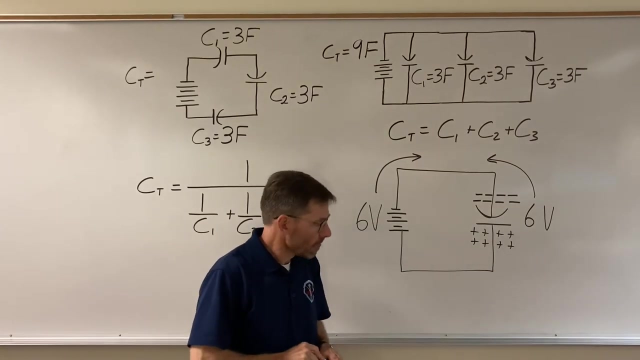 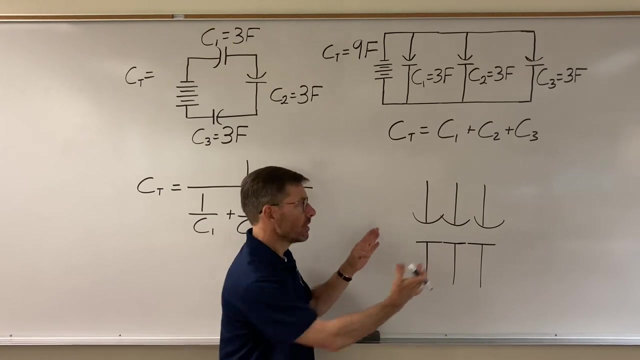 source. an equal charge here and another one there. I have more electrons So I'm going to stack more total charge. So three plus three plus three equals nine farads. The other way of looking at that is if I envision the three of them just pushed together, They're all getting the same. 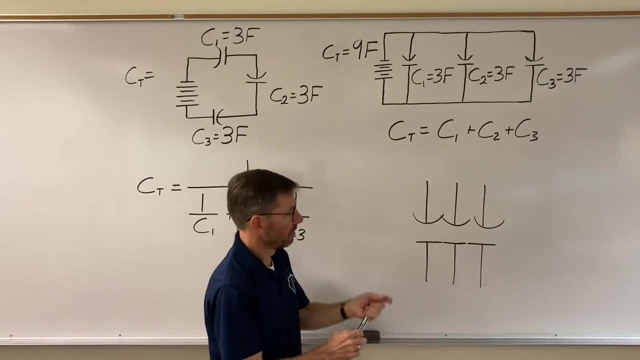 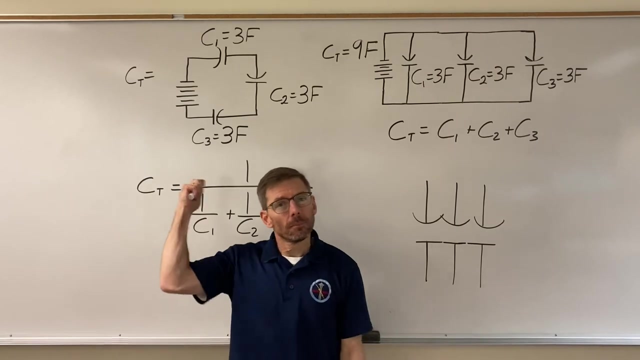 voltage on them. Why can't I just push them together? And does it look like the plates got larger, More capacitance. So I need a formula that yields a greater capacitance at the total than any individual branch. But what's happening on the series? 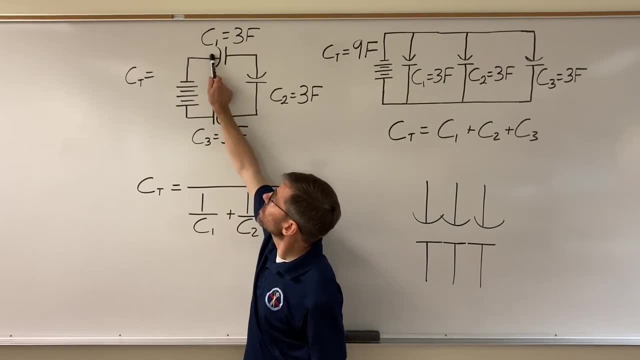 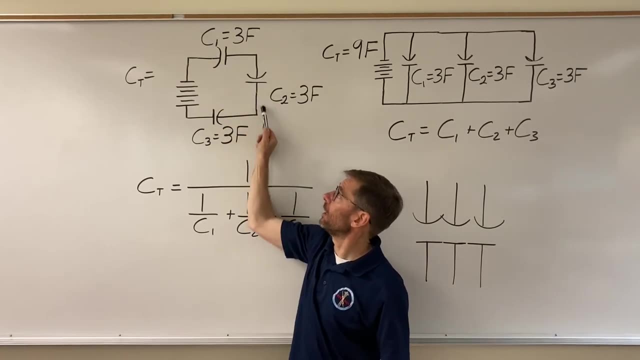 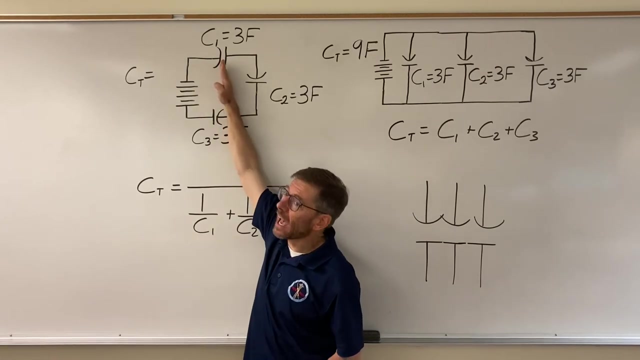 The voltage source is pushing electrons this way and they stack up here, repelling these electrons down to here. These guys repel these ones onto here and these ones get repelled and pulled together. So I need to get the voltage to be pulled by the battery. But we've got to work across this gap. 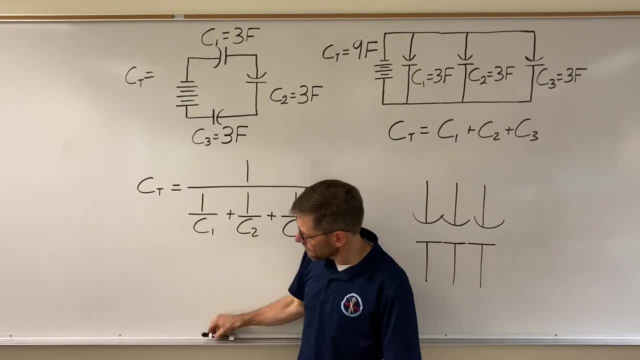 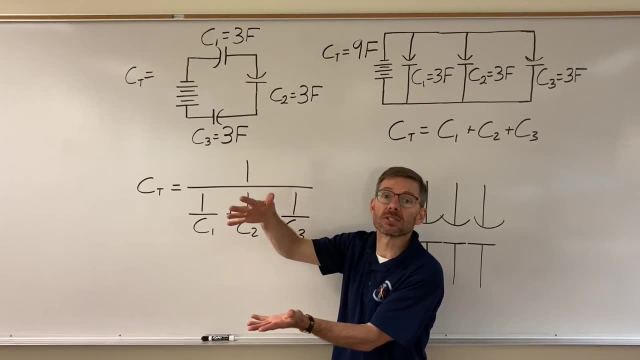 this gap got to work across this gap. What happened to my capacitance? as the gap between the plates increased, It got less. So that's the picture I want us to see here: that we're increasing the gap across the capacitor, And so I can't hold as much of a charge. It's harder to hold that charge as the electrons and the positives are further apart, So I can't hold as much of a charge. So I can't hold as much of a charge. It's harder to hold that charge as the electrons and the positives are further apart.